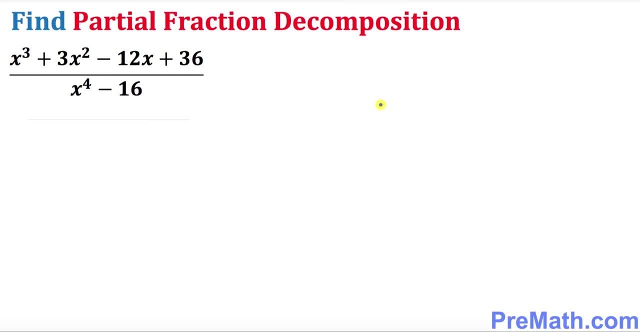 Hello again, everyone. In this video tutorial, we will be finding the partial fraction for this given example. Next step is to make sure that the degree in the numerator is indeed less than the degree in the denominator. Now let's focus on the denominator, this part. Okay, I want you to. 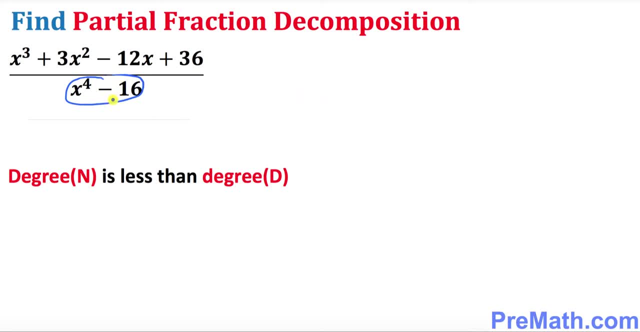 we're going to factor this one out. that can be easily factored. We will be using this fact. So this is the difference of two squares. we will be using this formula. So let's go ahead and put it down this: x power 4 minus 16, right up here. Let's manipulate this thing a little bit. I'm. 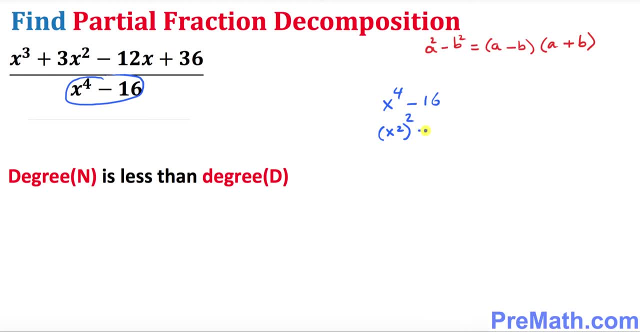 going to put down x power 2 and then power 2 and then 4 power 2, that same as 16.. Now I want you to make sure that the x power 2 could be treated like an a and 4 is like a b. 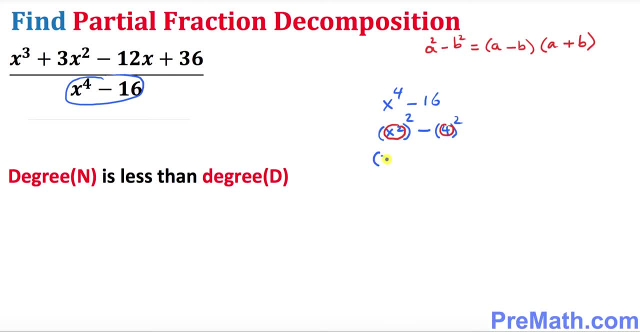 Then this whole thing could be written as x square minus 4 times x square plus 4.. Isn't it That's nice? Now I want you to look at this box over here, Isn't it? this part? this could be be factorized, So the possible factor is going to be: for that one is going to be x square. 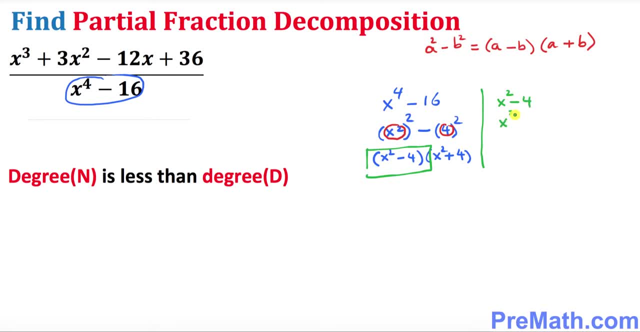 minus 4 could be written as x square minus 2 square, which is same as x minus 2 times x plus 2.. So I want you to just put it down over here: x minus 2 times x plus 2 times x square plus 4.. 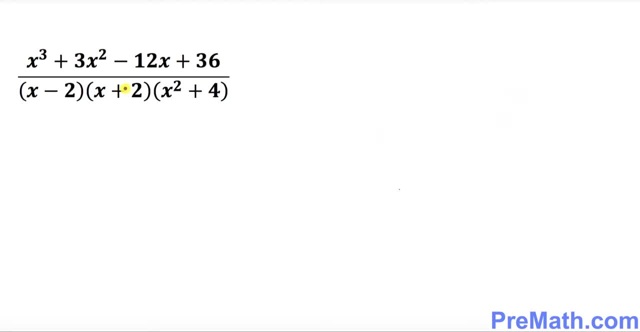 Piece of cake. Thus our rational expression can be rewritten as the factors at the bottom like this thing. Let's go ahead and set it up for partial fraction. So, at the bottom, just make sure that there are two linear factors and this is a quadratic factor. Whenever you have a linear 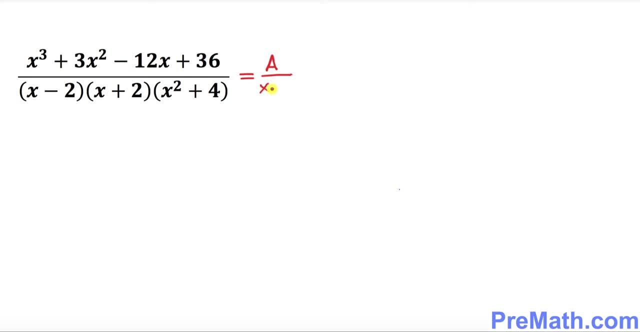 factors. you just simply put down a over x minus 2 plus x square minus 2 times x square plus 2.. So it is quite easy. I'll just put at the bottom and you will see, that the condition of our next should be that the number of bullets that you can put at your 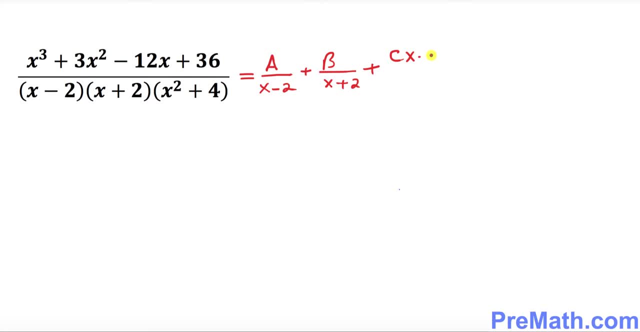 position should be equal to a vector of return first used as the positiveator, Which is kind of a bit tricky, right? Okay, both of these three are UE and we know the result very well. OK now. now we will look for Rome. 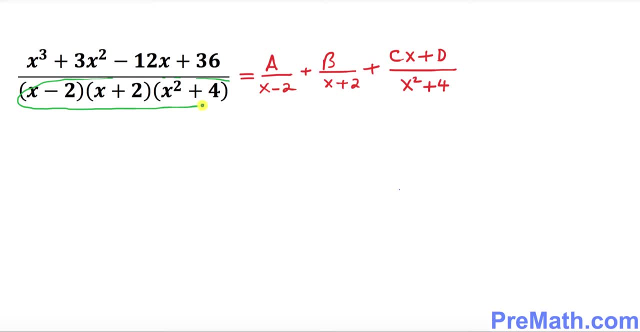 Right, So here's Rome part. whatever over here across the board, we're going to multiply, so let's go ahead and multiply x minus 2 times x plus 2 times x square plus 4. we're going to do the same thing for this one as well: x minus 2 times x plus 2 times x. 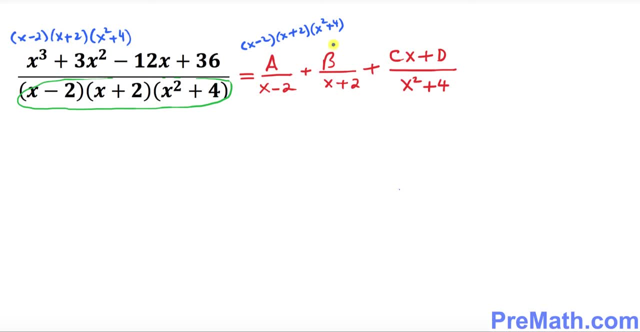 square plus 4. likewise, x minus 2 times x plus 2 times x square plus 4. and finally, for this one as well, x minus 2 times x plus 2 times x square plus 4. now you can see one thing: this thing cancel with this one. this cancel with this one, this. 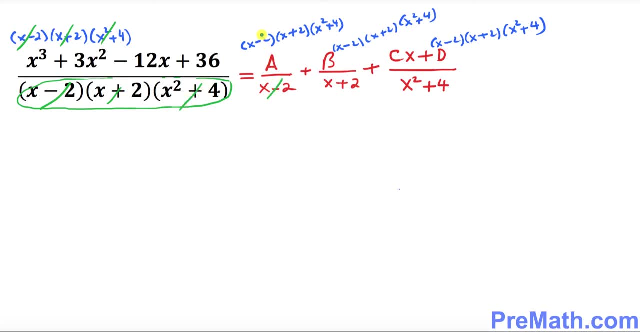 is done with this one. likewise, this is canceled with this one. this is gone with this one. this is gone with this one. and we ended up with x power 3 plus 3x square minus 12x plus 36 is equal to, on the right-hand side, a. times x minus 2 times x underneath for chase is equal to 1 root 3 times 1 times x plus 4 he àz. Second. Well, was at the start, if you look at these terms, that we're looking at the head and 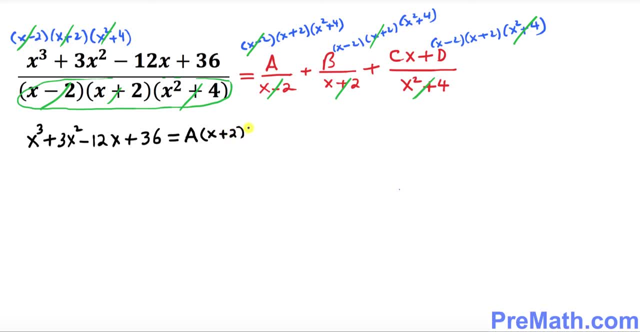 times x plus 2 times x square plus 4 plus b times x minus 2 times x square plus 4.. And finally, cx plus d times simply x minus 2 times x plus 2.. And we want to call this whole long equation as our equation number 1.. 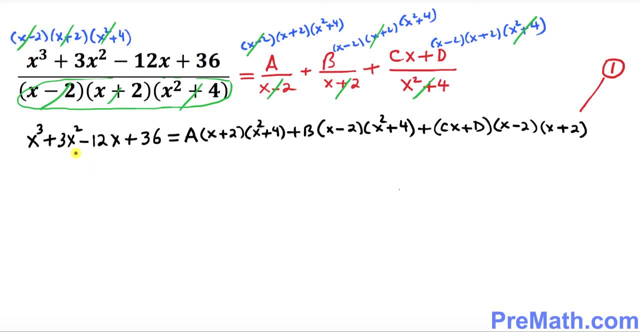 Just keep in your mind. So the next step is we want to find the value of a, b, c and d, And for that one we will be using a really simple kind of trick. Here is the simple trick: Whatever you have, the linear factors x minus 2 and x plus 2, I separately set them equal. 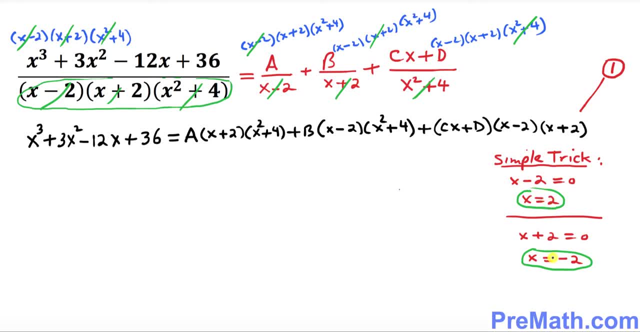 to 0, and then x turns out to be equal to 2 and negative 2.. This is what is going to help us. So I'm going to say: add x equal to 2 first, Like from here, Plug it in. This is our equation number 1.. 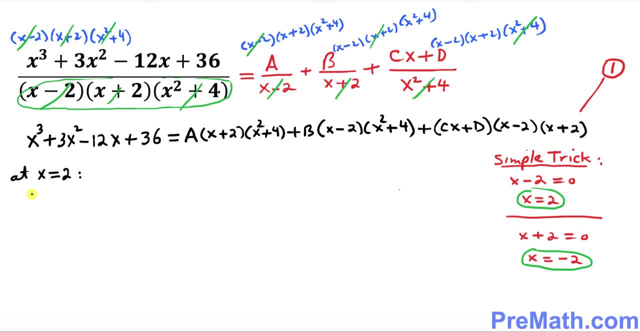 So once you plug it in, what's going to happen? So that's going to become 2 power 3 plus 3, 2 power 2 minus 12, times 2 plus 36, equal to a times 2 plus 2 times 2 square plus 4.. 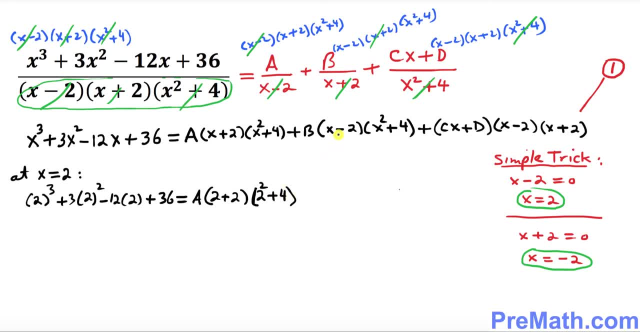 And when you look at b part over here, you see 2 minus 2, that's going to give you 0. So we know the whole thing is going to become 0. And likewise, in this next term, 2 minus 2 is going to be 0. 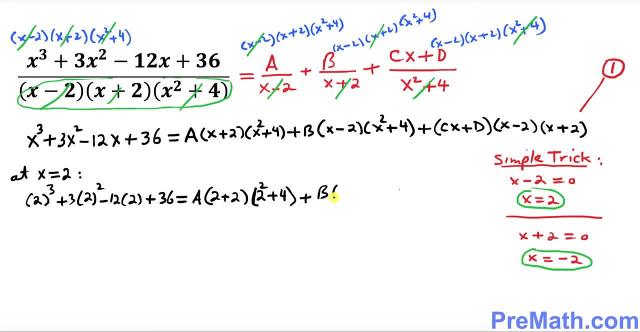 So that means I can write b times 0 plus cx plus d times 0.. Now we're going to have to do the whole thing again, So we're going to write 2 minus 2.. So that's going to be 0. 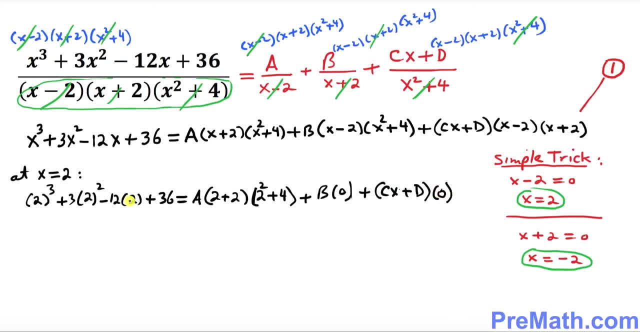 We're going to write cx plus d times 0.. so once you simplify that thing on the left hand side, this turns out to be 32 equals to 32, a, and this is 0 and 0. don't worry about that thing. so a turns out to: 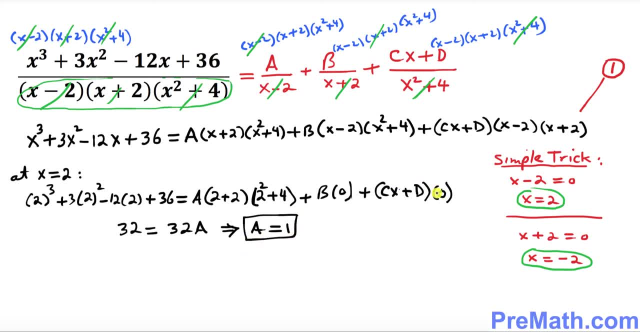 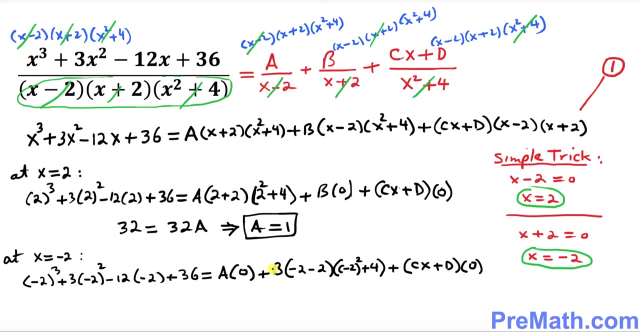 be equal to 1. likewise at x equals to negative 2. as you can see from here, we're gonna plug it in our values in our equation number 1, after plugging in x equal to negative 2. we got this whole thing and just once again make sure that in our equation number 1, a is equal to 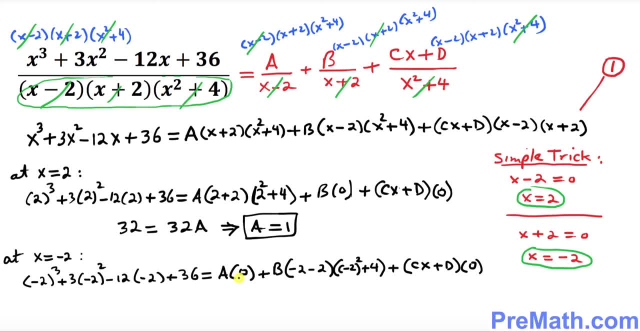 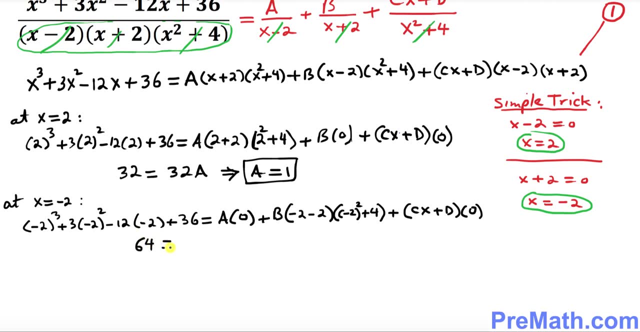 see right now, negative 2 plus 2 is 0, so no wonder I put down 0 over here. and likewise negative 2 plus 2 is 0. so if we simplify this thing, that's gonna give you how much on the left hand side is gonna be a 64 equal to negative 32, b, which tells us that b equal to simply. 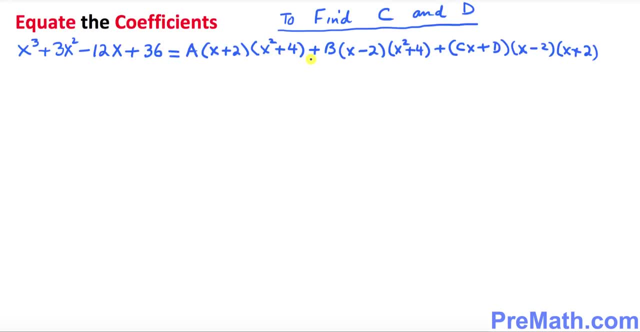 negative. 2 plus 2 is 0.. Now we need to find c and d, and the only possible way to find c and d is to use this method that is called equate the coefficients. so you're gonna watch and see how I'm gonna do that one. so the 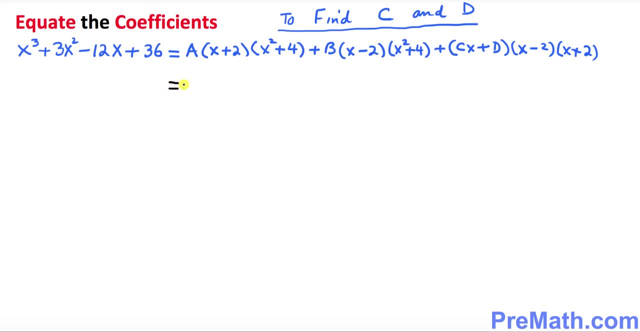 very first thing, what I'm gonna do is, on the right hand side, I want you to multiply these polynomials. when you multiply these one, what you're gonna get X, power, 3 plus 4, x plus 2, x, square plus 8. likewise, I want you to put down b and multiply. 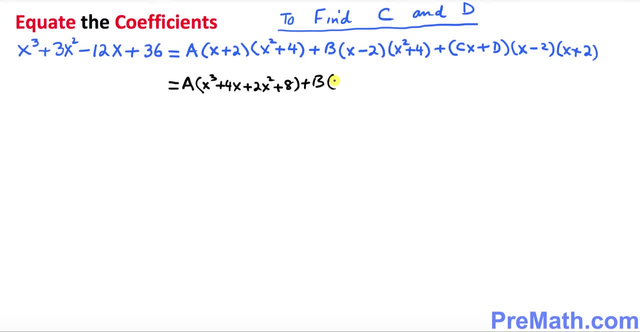 these one. I'll just distribute these one. how much you're gonna get this is you use a foil method: x power 3, x power 3 plus 4x. all right복, you'll get what I'm gonna get this way. I think she said so, how we do it this way. if we take 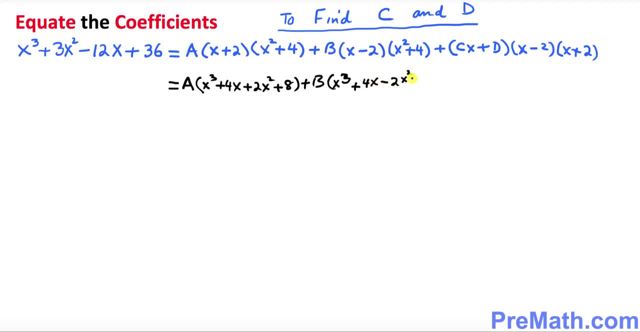 the one that below these, all the way till the upper, others below out, all the way all to the ends, and you'll solve it. how you'll solve it? okay, this was it, basically, because we probably minus 2x square, minus 8, and then plus, you just put down cx plus d time this is going to give you. 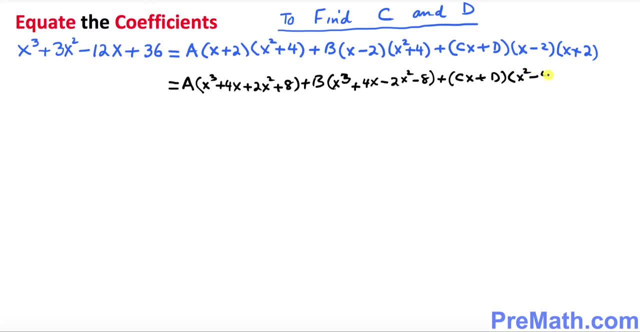 x square minus 4. do you see that one? so let's go ahead and just distribute this thing, and this is what we're going to get. you just distribute and we're going to get, and, after the distribution, this is what we got. you can see that thing. now the next step, what I want you to do is go ahead. 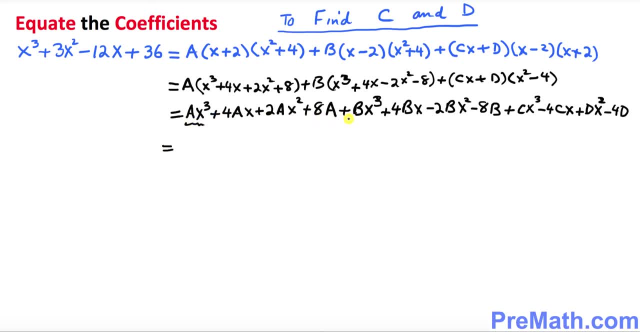 and look for x power 3 terms: x power 3, x power 3 and x power 3. I can combine these one. I can write down what a plus b plus c times x power three, isn't it? now? I want you to look at this: x squared times this: 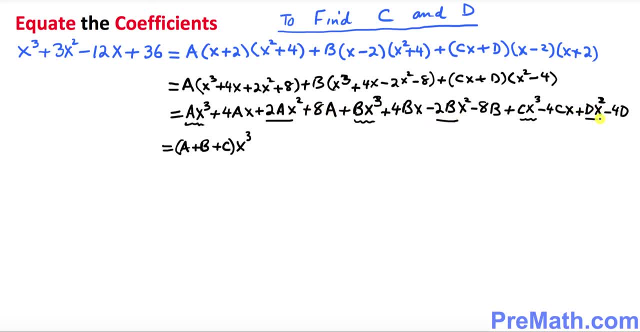 is x square term and this is x squared terms. I'm going to put it together. I can write: plus 2 a, minus 2 b, plus d times x squared. now I want you to look at x term, which this as x is you are considering when you identificatEthe 키. no matter, 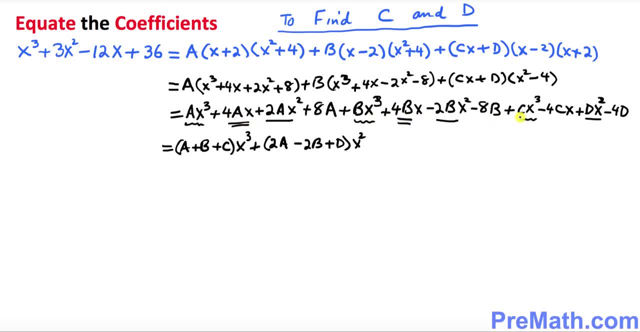 term and we have a this X term and this X term I'm going to write down as plus as 4a plus 4b minus 4c times X and finally plus constant terms, which is 8a minus 8b minus 4c. 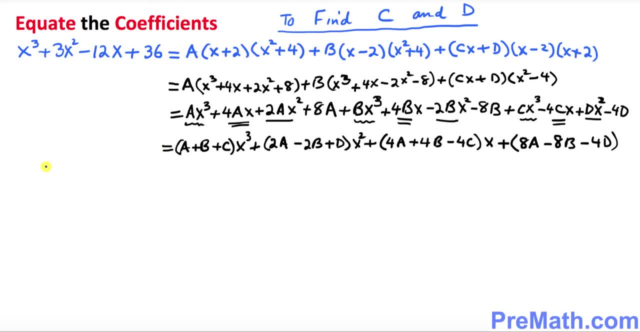 d. These are our constant terms, and on the left hand side I can write x power 3 as 1 x power 3 plus 3 x square minus 12 x plus 36.. Now in this step we're going to equate or compare the. 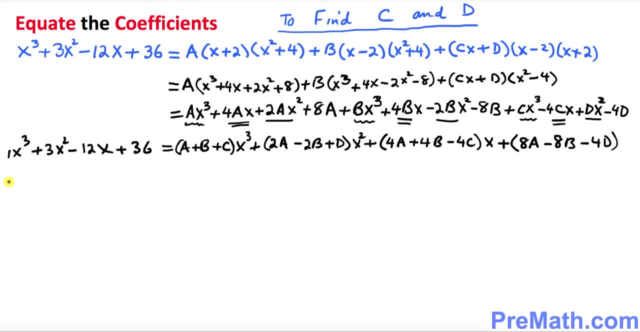 coefficients along with this thing. First, I'm going to go ahead and look at x power 3, x power 3 terms. Look at x power 3 term, what it's going to give you on the left hand side. The coefficient for x power 3 on the left hand side is 1 and on the right hand side it is simply. 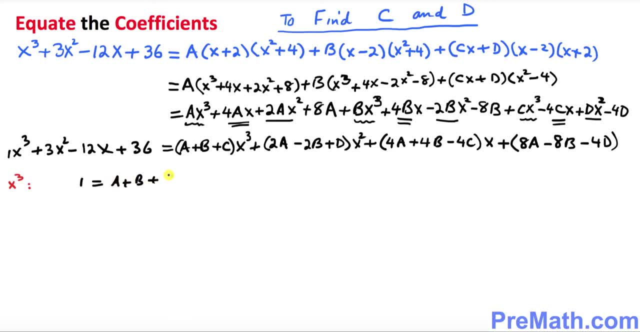 a plus b Plus c. Now, likewise I want to do for x square term. I'm going to do this one and that's going to give you what. on this side is a, 3, the coefficient, and this side is 2 a minus 2, b plus d. 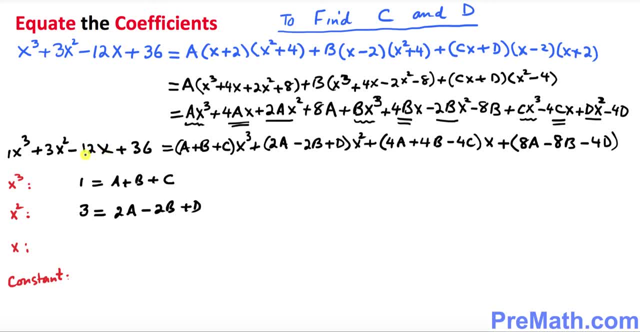 For x variable, the, on the left hand side, the coefficient is 2 a minus 2 b plus d. Negative 12. equals to, on this side, is 4 a plus 4 b minus 4 c. and for constant on the left hand side is just simply 36. equals to, on this side, is going to be 8 a minus 8 b minus 4 d. 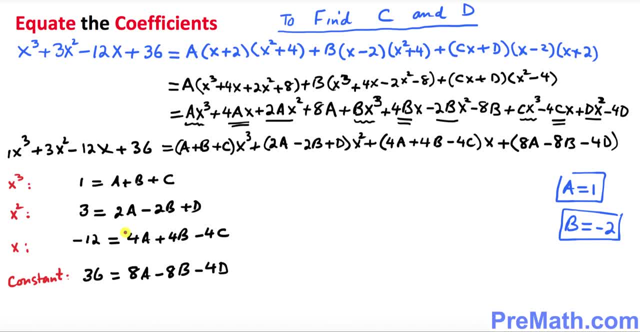 So thus we got all these 4 equations, and we already know that a equals to 1 and b equals to negative 2.. I want to call this equation 2.. I want to call this 3.. This is 4 and this one as 5.. 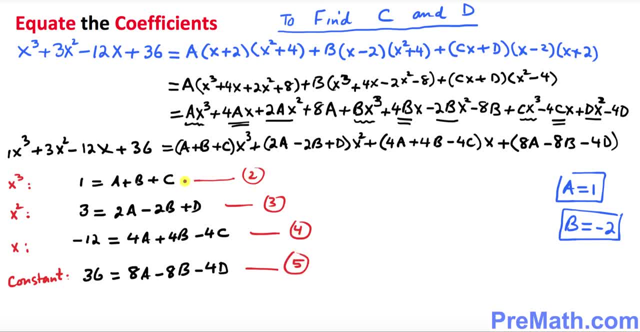 Now I want you to look at this equation number 2.. We know that a is a is what, a is 1 and b is negative. 2 c is going to. we can easily figure out from here that is going to give us what. 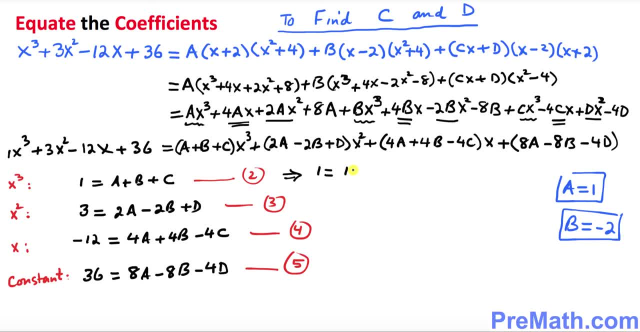 So 1 equals to a is already 1 plus b is negative, 2 plus c, And if you simplify, you're going to see that one that c, turns out to be simply 2.. So now we're going to focus on this equation number 3..